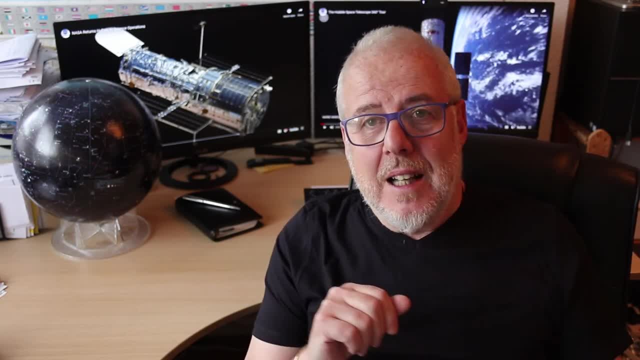 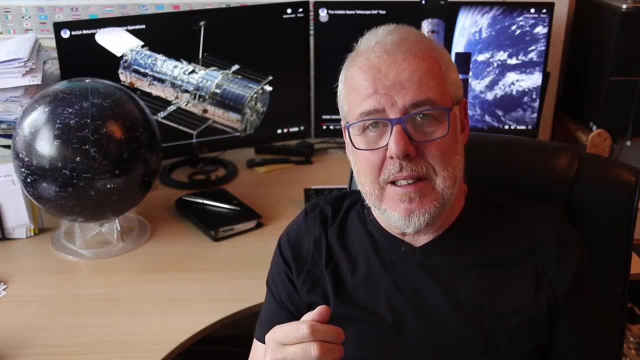 Hi, folks. Well, finally, astronomical darkness has returned to where I live in the UK. At the moment, though, it's only an hour or so, but in the next couple of weeks it should be sufficiently long for me to get out and do some serious imaging, and I can't wait. 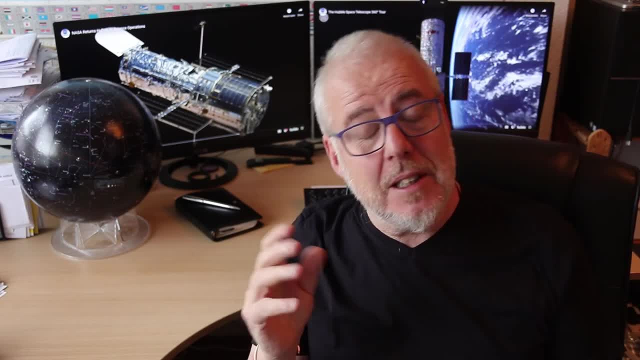 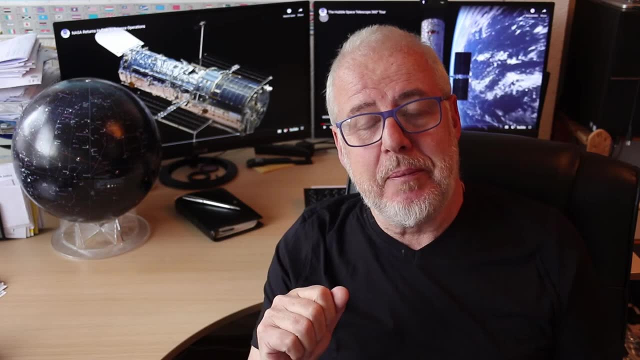 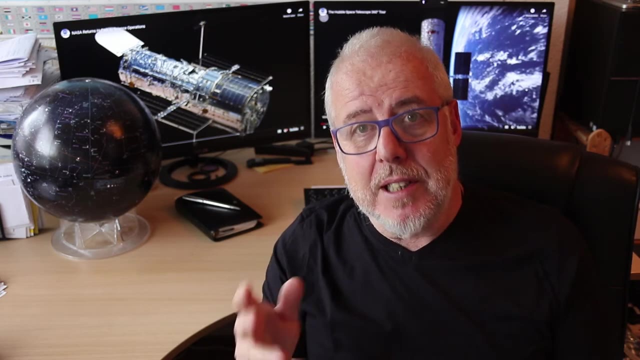 But meantime, what I'd do for a bit of fun and interest is: I thought I'd access the data from images relating to the Hubble Space Telescope. You can do this from an internet site called the Hubble Legacy Archive. It's free to use and you can download images and process them using your normal workflow. 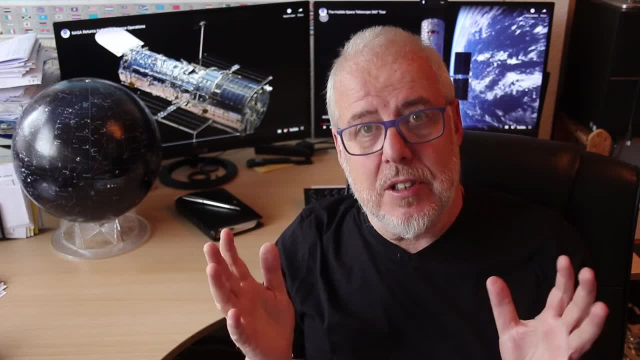 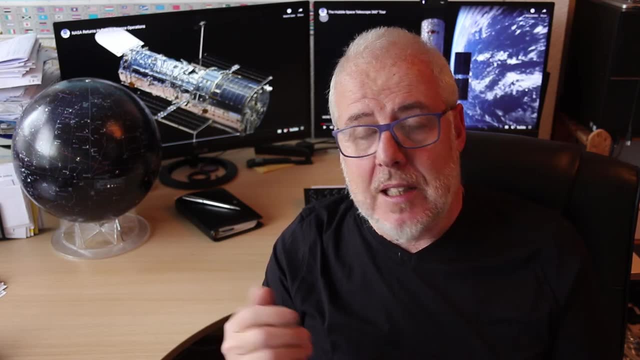 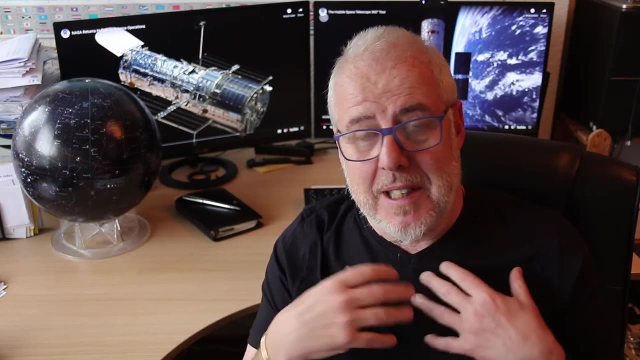 As I say, it's very interesting. You can actually access images that haven't been published before, that you perhaps haven't seen before, And it's also a good chance to practice your processing skills. If you're like me, they certainly need improving. 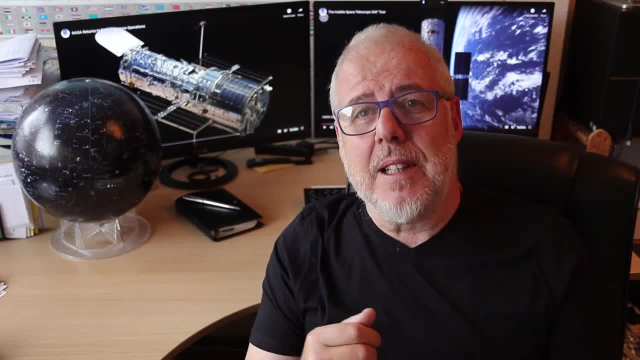 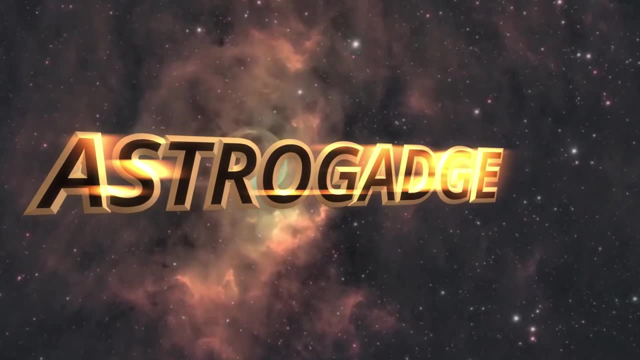 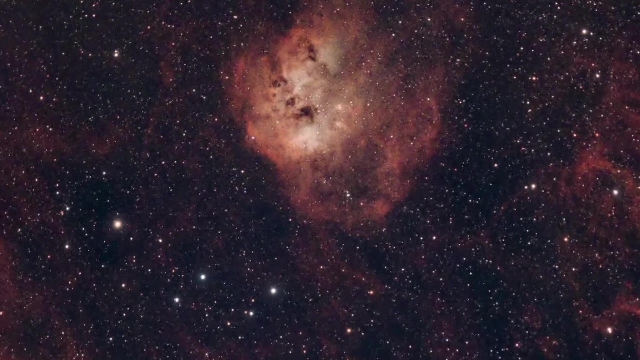 So let's go and have a look at the Hubble Legacy Archive. I'm Dr Ray and welcome to AstroGadget. Okay, so here we are inside the Hubble Legacy Archive, which is the name set for the Gigabyte. 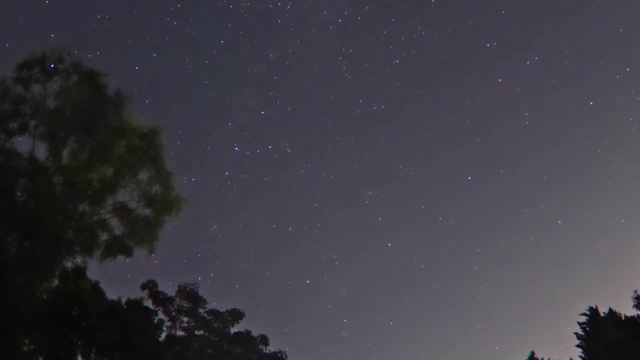 And on our screen you can see two of the Hubble Space Telescope's latest models. You can see that two of them were built with the help of my friend, Dr Ray and Dr Ray, and they're on their way to the future. 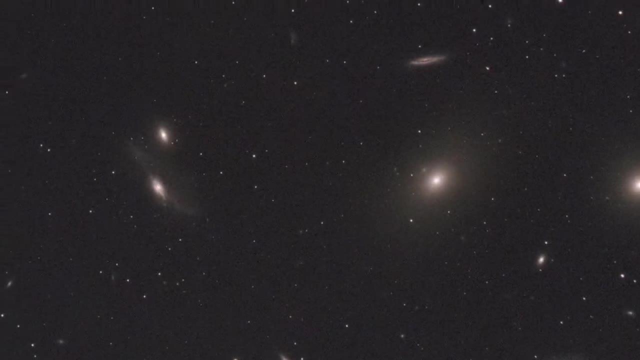 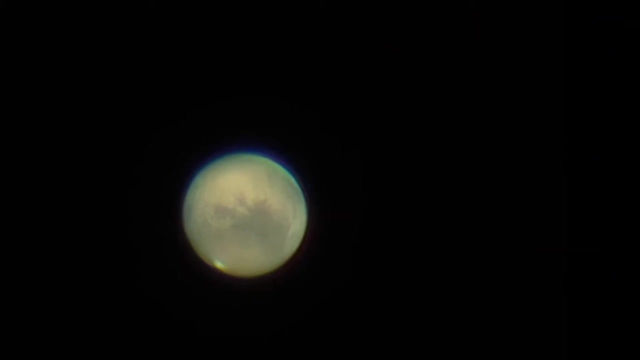 But they were never made, So here's how we can access them. I'll show you how to do it in a minute. You can go here and see that a couple of images are there. You can also see the Hubble Legacy Archive, the Hubble Space Telescope. 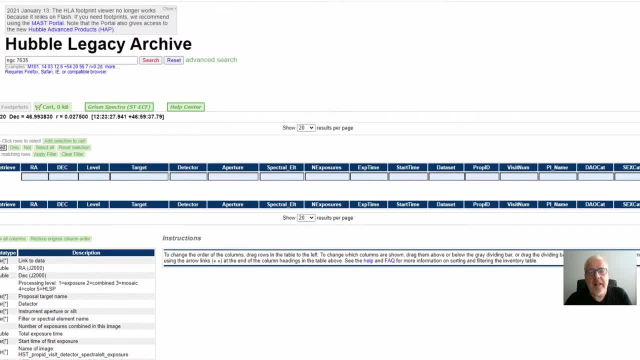 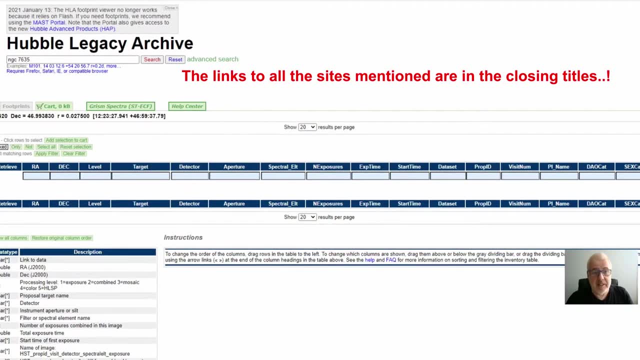 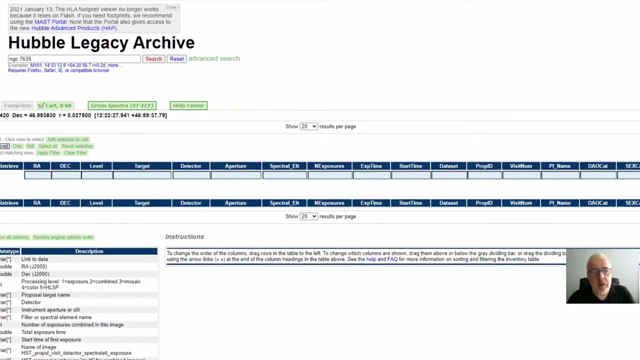 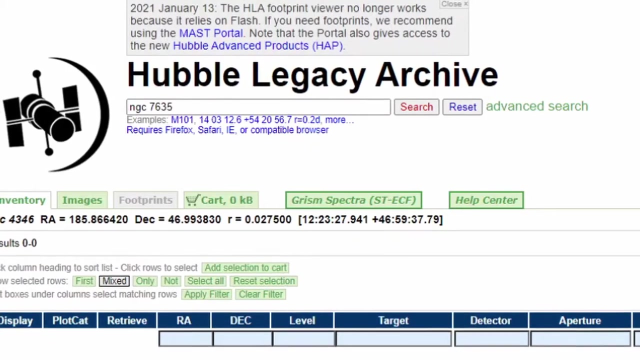 You can also see the Hubble-Legacy Archive Archive which, as the name suggests, is simply an archive or database, as I said, of various images taken by the Hubble Space Telescope. So what I've done is I've put in the search window here NGC 7635,, which is the bubble nebula, and I want to 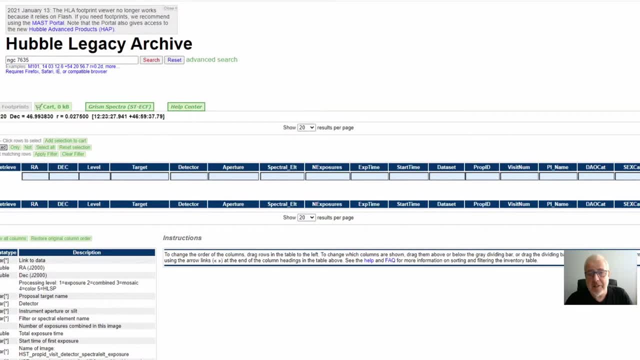 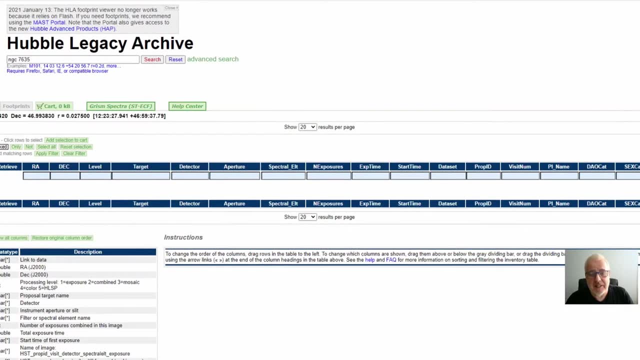 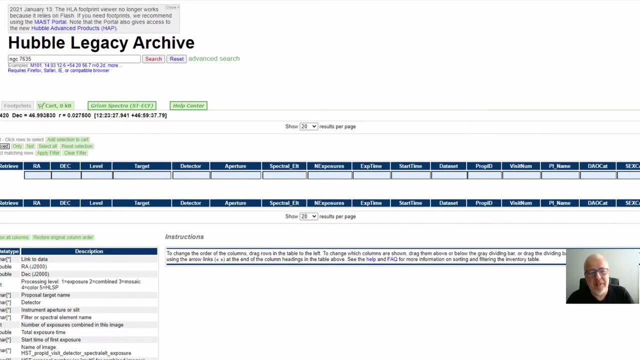 show you the images taken by the Hubble compared to my meagre ground-based efforts, for want of a better word, It's just mainly out of interest, just to show, if at all needed to be shown, what the difference is, but also quite interested in seeing. 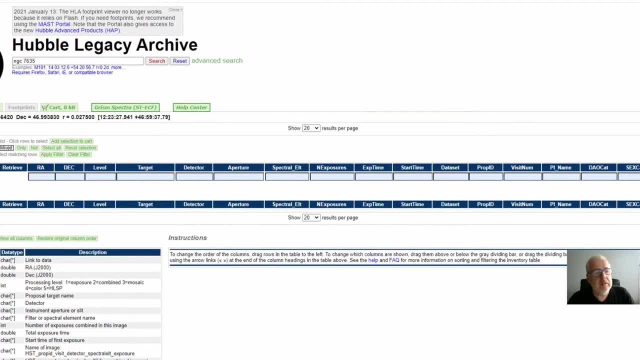 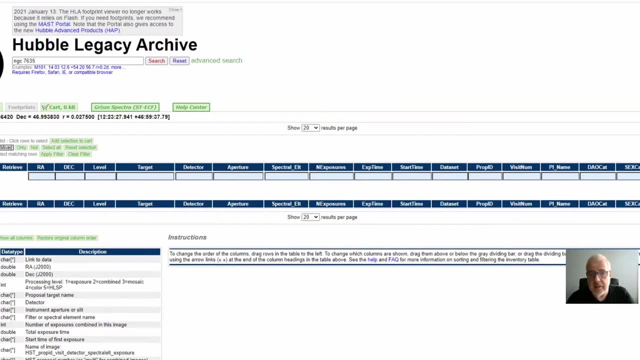 what detail this can bring out as well. So, as I say, I've inputted the name of it. You can use coordinates as well if you like, but it's simpler just to use the usual designations. So, again, we will simply press search and. 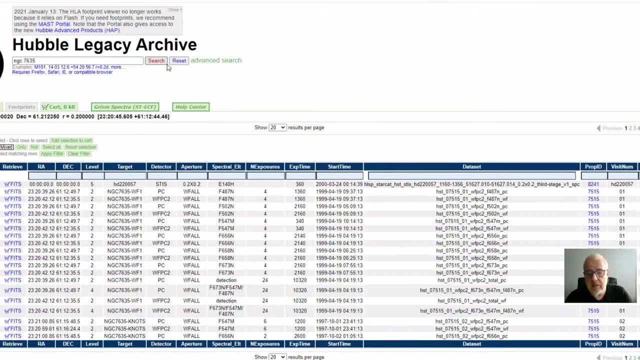 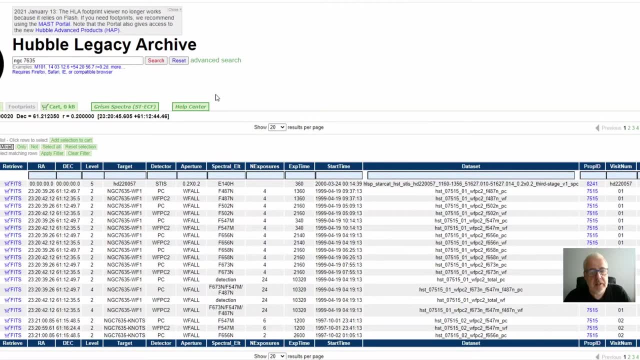 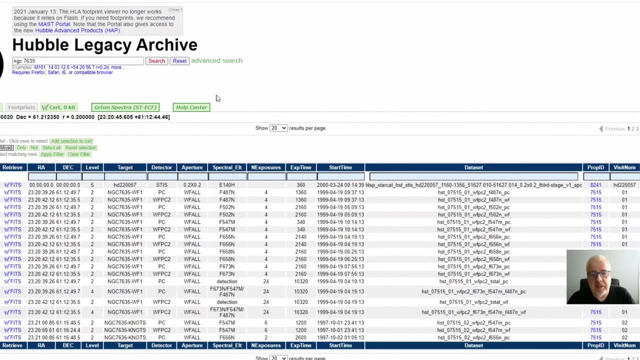 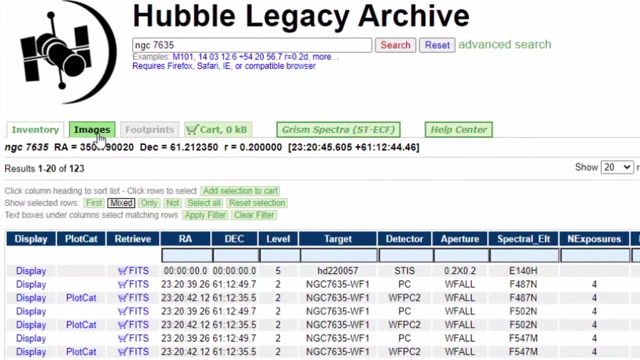 uh, here we have a whole load of files that relate to the bubble nebula. So what's good about this is actually there are little previews of the examples of the image or little thumbnails that can help you decide what it is you want to download, and to do that is simply go into this tab here and up it comes. So 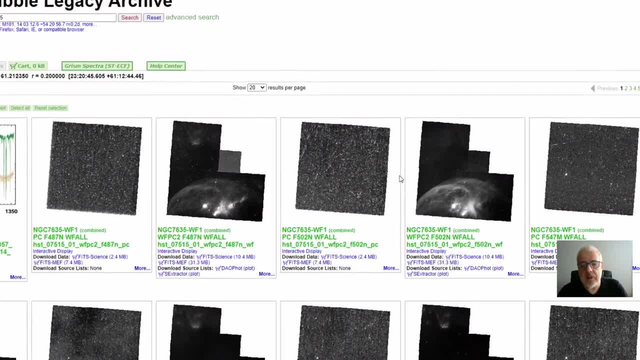 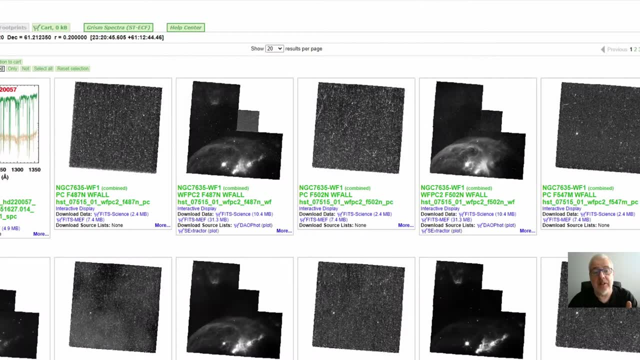 as you can see, there are a lot of images taken by the Hubble Space Telescope and you can see there are various files, various images, uh, that have been taken by the Hubble. Before we go any further and download some of these images, it's worthwhile to say a little. 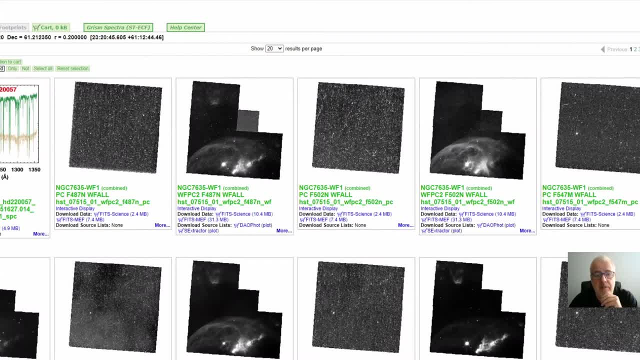 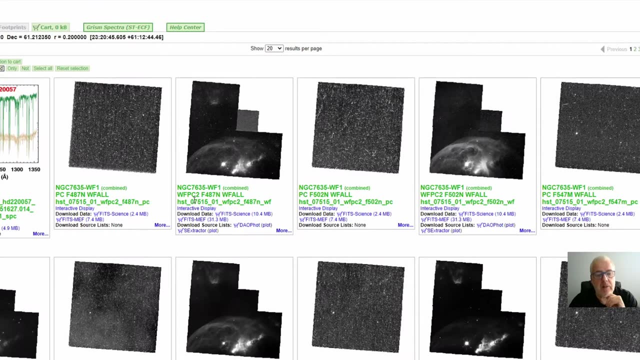 bit about the file names, the nomenclature of the different files. So let's look at this one here, for example. Now this is the file name here. So what this is telling us is this number here is what's simply called the proposal number, in other words, the project number. so, for example, 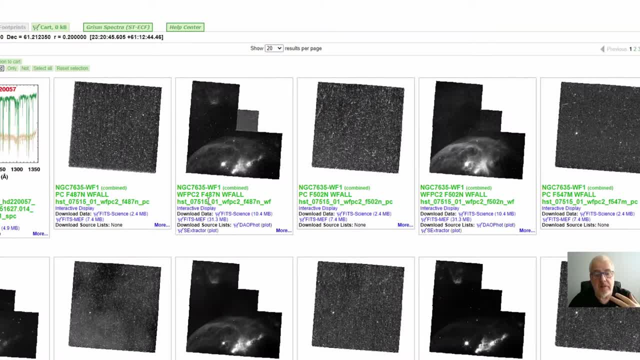 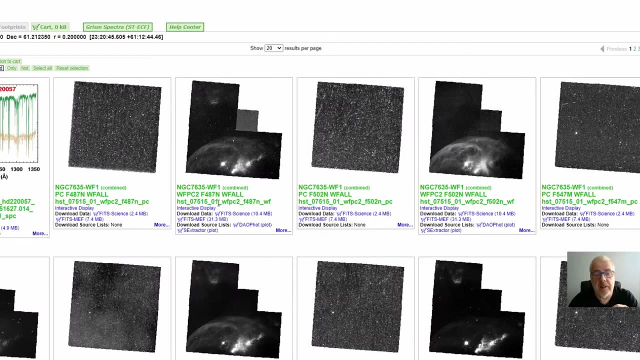 if they're taking a picture of this particular region of the bubble nebula, they would simply refer to it as 07515, a project number by any other name. so that's a particular project number. and the second number is the number of times they've actually visited or recorded this. 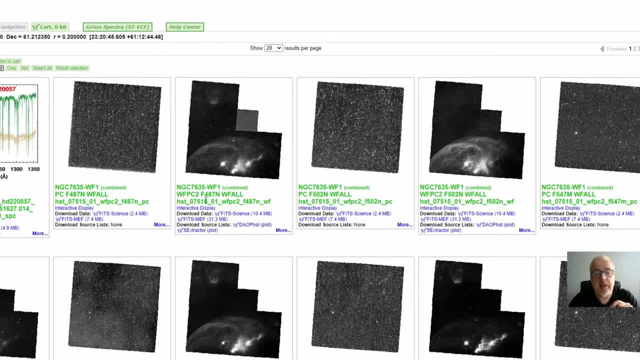 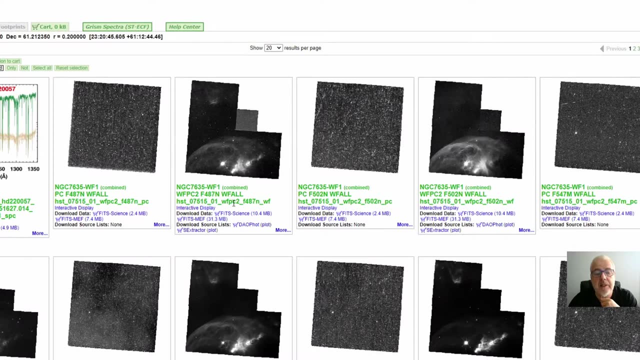 particular project, so in this case, this particular project. this was the first time they'd actually imaged this particular part of the of the bubble nebula. the next, the next part. here wfpc2 stands for, while stands for wide field planetary camera 2.. now, that's a particular camera that was installed. 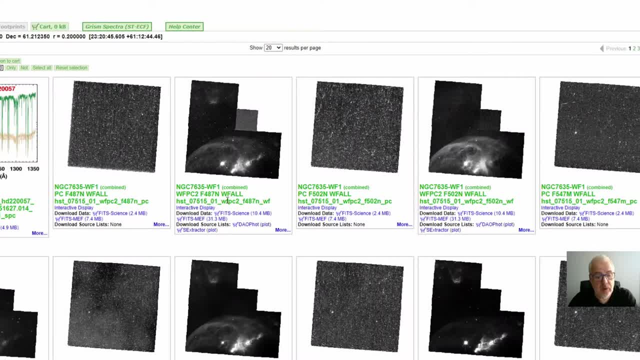 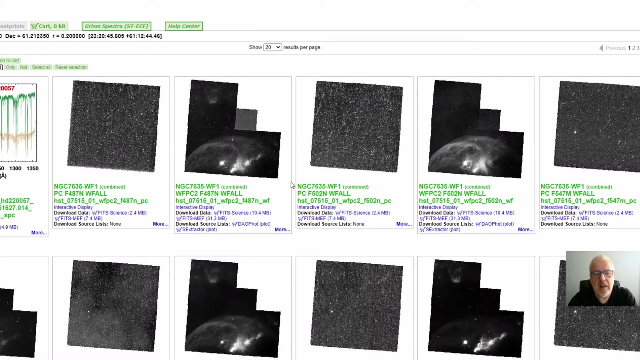 on the hubble telescope in 1994, when it was replaced in 2009 by the wide field planetary camera 3.. and one of the things about the the wide field pc2 is it takes a sort of mosaic in this almost stealth bomber sort of shape, which is a little bit- well, not annoying, but it just means you have to. 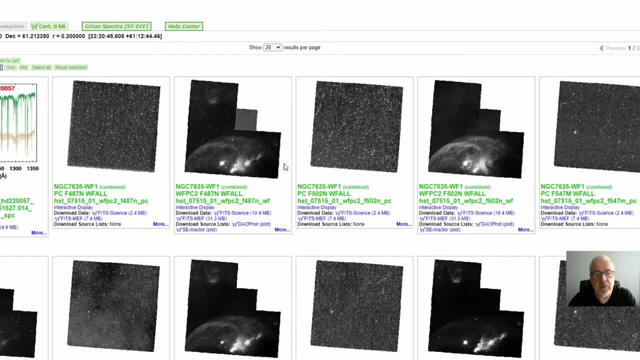 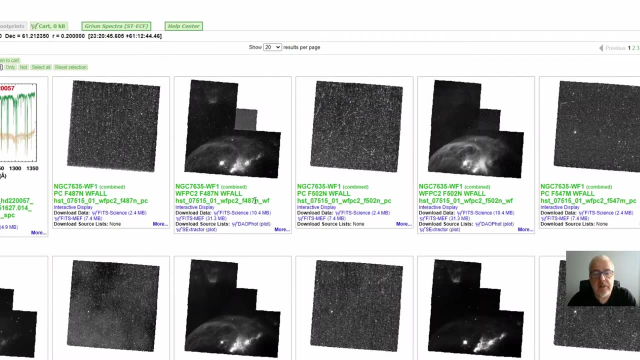 play about with the crop to to get, to get the image, uh, the way you want it. uh. wide field, uh. planetary camera 3 is more of a sort of square, um, more of a square sort of frame, um. the next number is, uh stands for the filter they've used. so this, this particular filter, this particular image was taken with a. 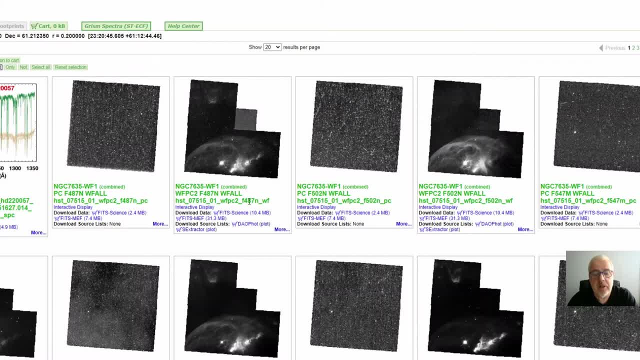 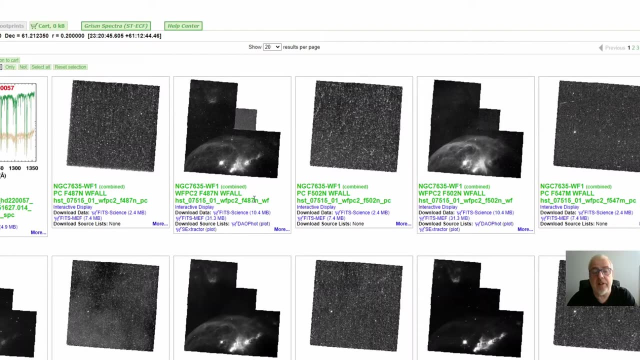 filter of 487 nanometers and the n stands for narrow band, so it's a narrow band filter. okay, the other designations you can get are w, which is uh, they refer to as wideband. we would probably refer to, as amateur astrophotographers, as broadband. so that's just so, it's basically. 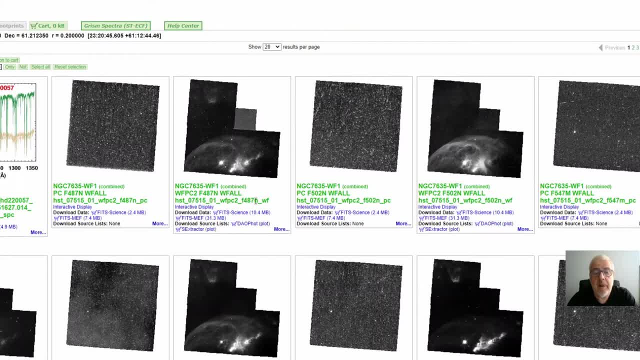 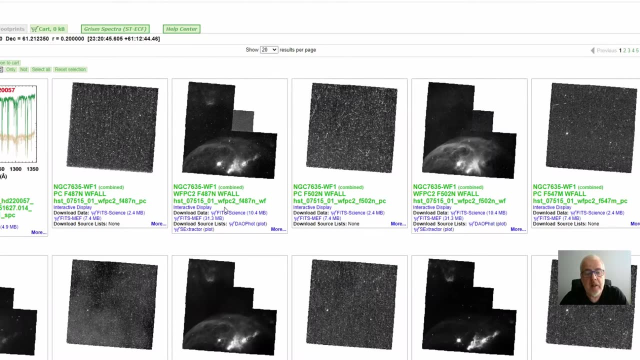 a 487 nanometer filter and it's. it's a narrow band filter and again, the wf just means it's a wide field camera that's been used. that that's how the uh nomenclature is used. now, if you're going to download um a number of files, say for red, green and blue, um integration. 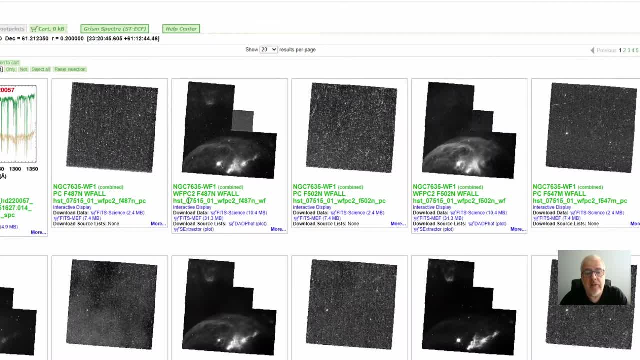 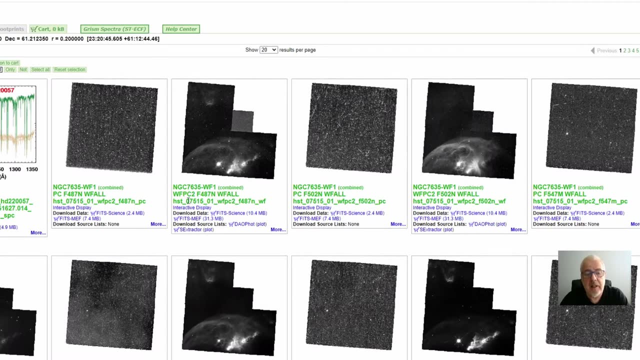 then you're best going for the same proposal number and visit number. if you don't, there's a chance that the alignment might not be exactly the same and cause you problems later. so it's always best going for um a number of files, images relating to this, these numbers here. so if we go along here we can see this is the same. 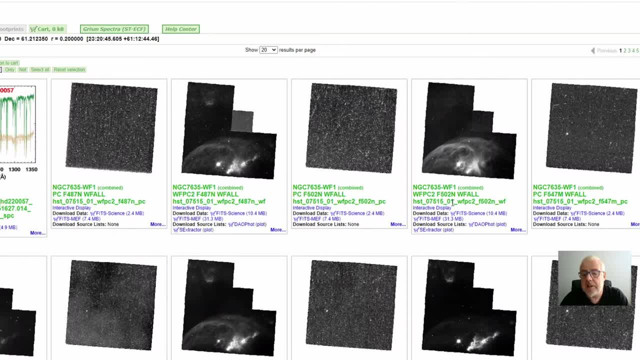 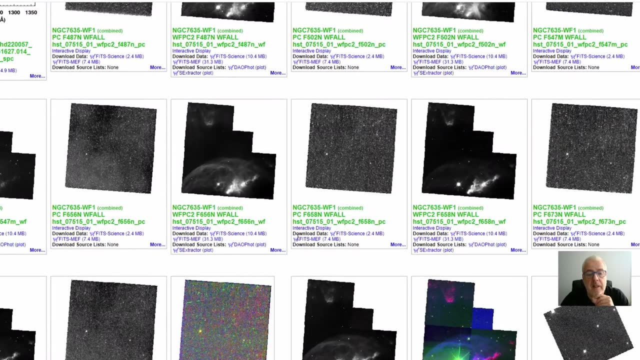 project or proposition number and it's the same visit, but this time it's the same camera, but this time they used a filter at 502 nanometers. okay, and likewise, if we move down again, we can see that again the- uh, the same project number, the same visit number, but again it is a, again a different. 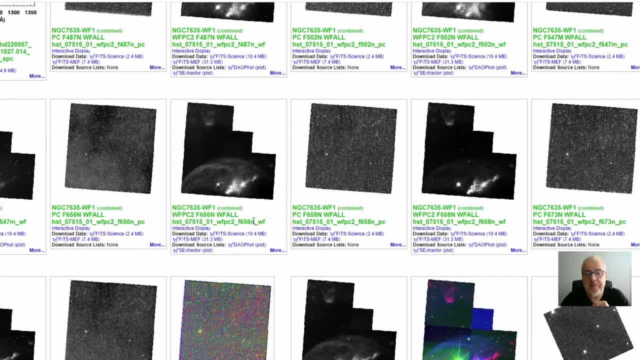 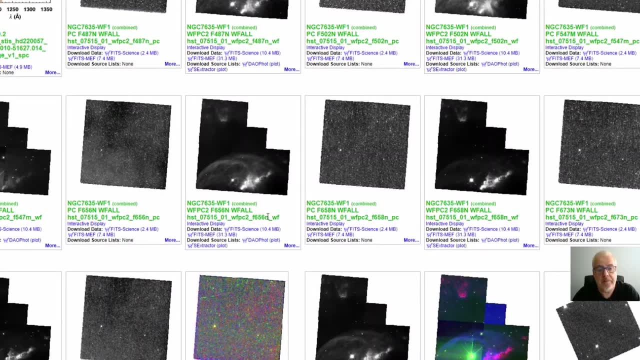 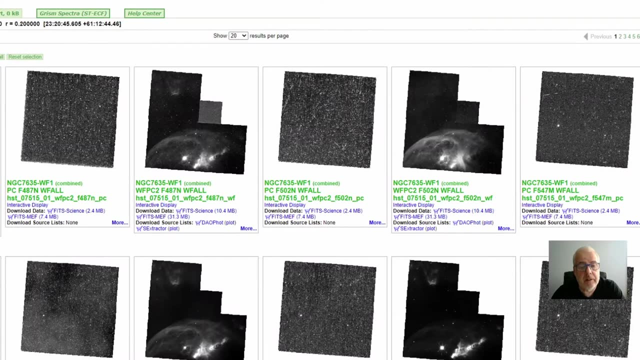 filter: 656 nanometers narrow band. so these are the, the three files i'm going to download that correspond to red, green and blue. to download these files, it's it's pretty straightforward, uh, you simply have to click on on the, the source that you want. now, uh, for for our purposes, uh, it's. 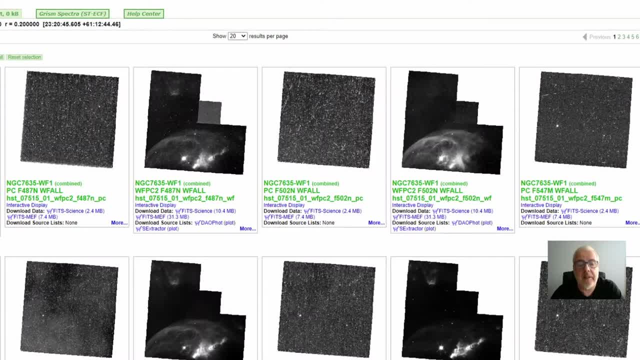 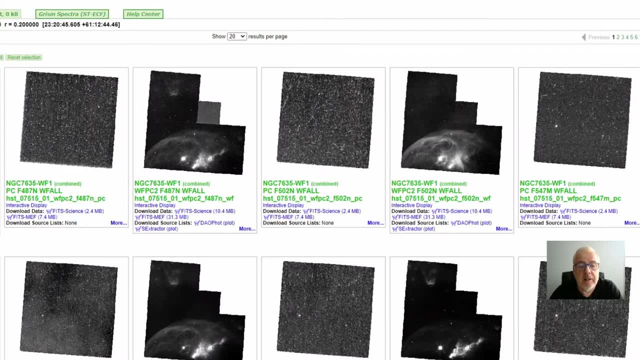 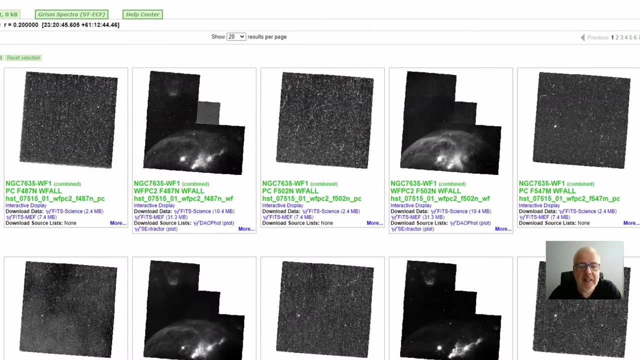 the science fits that we want it's in the fits format. uh, uh. you can download other source files, but they contain a lot of information that really isn't that well of interest, to me at least, uh. but if you're curious, by all means download them, and 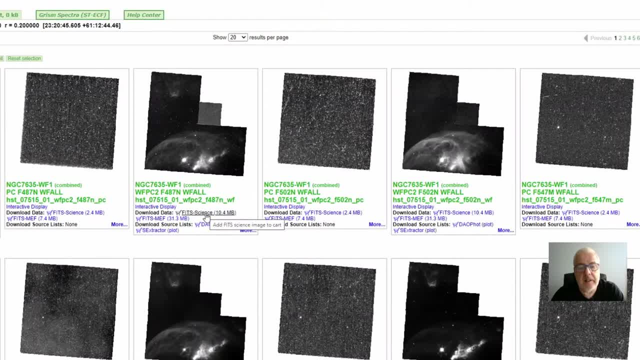 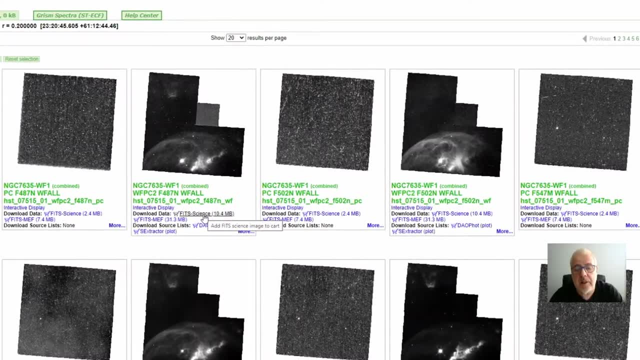 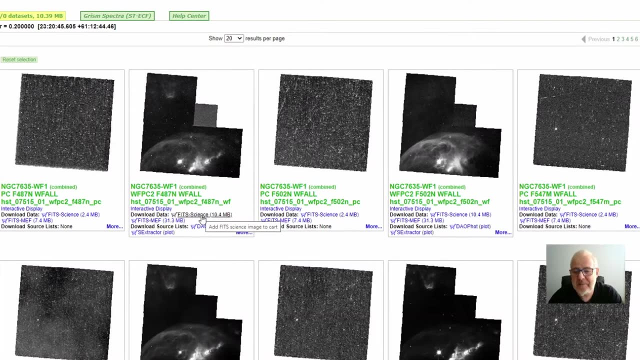 and see what's in them. but for imaging, dead easy. just click on the science tab to select it and you can see it's added to cart. don't worry, you're not going to get charged. okay, there's no charge for this, it's just a cart. the next file we're going to select is it? 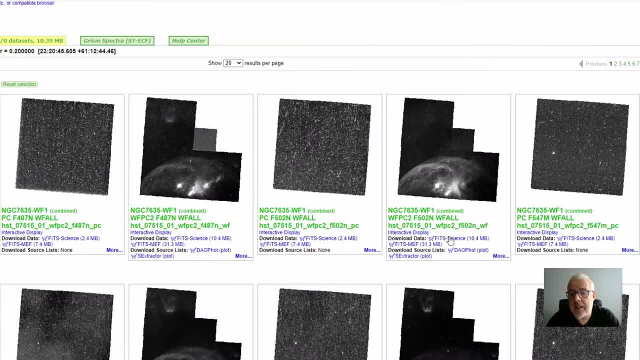 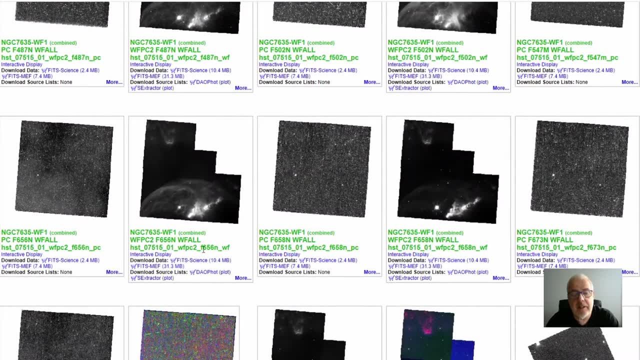 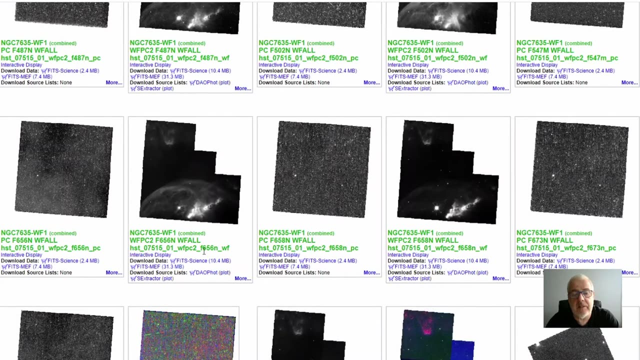 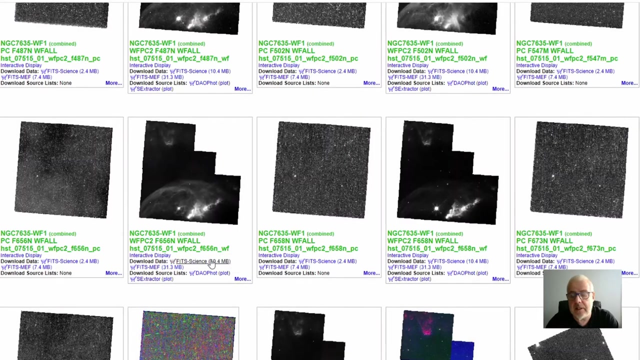 is using the 502 nanometer filter, and again, select that. and the third one we've decided to go for is, uh, again the same proposition number, same visit number, uh, same camera, but it's using 656 nanometers um filter, urban filter, and again we're going to, uh, just add that to the cart once they're all um. 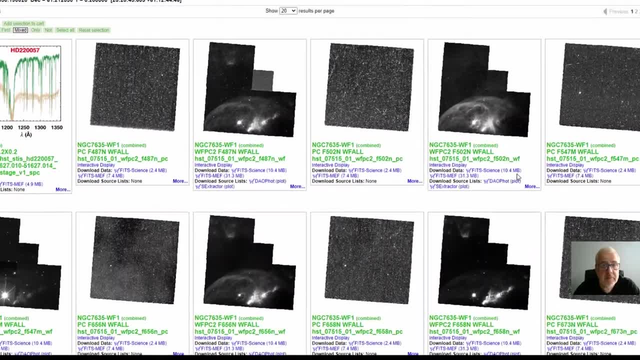 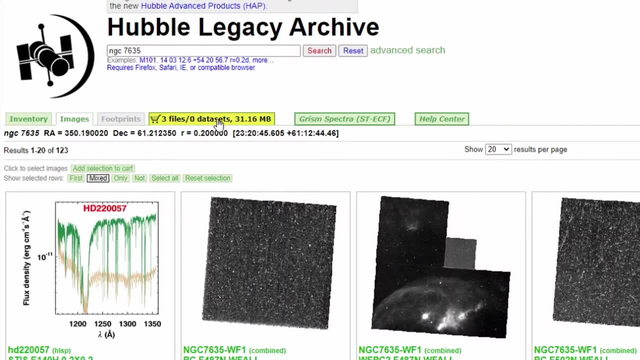 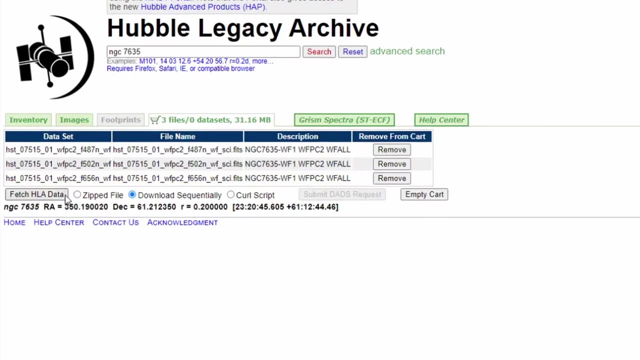 selected and added to the cart and you just simply scroll up. you'll simply see your cart- as i say, you don't have to pay for it- where your files are, you simply click on that and there's the files that you've selected. now you've got different options here. i i prefer the zip file. 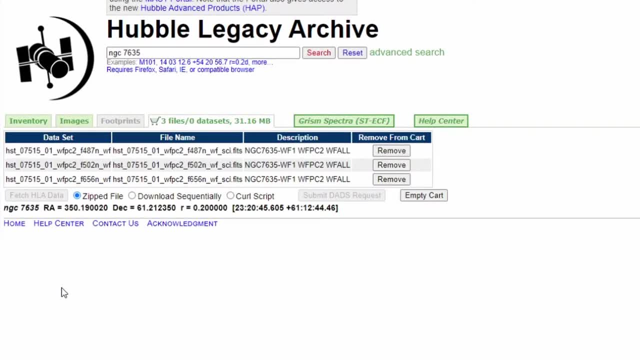 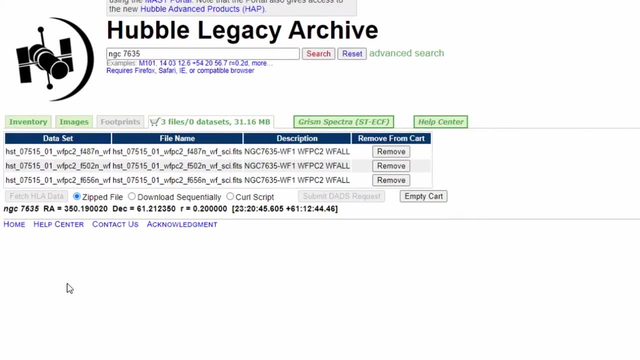 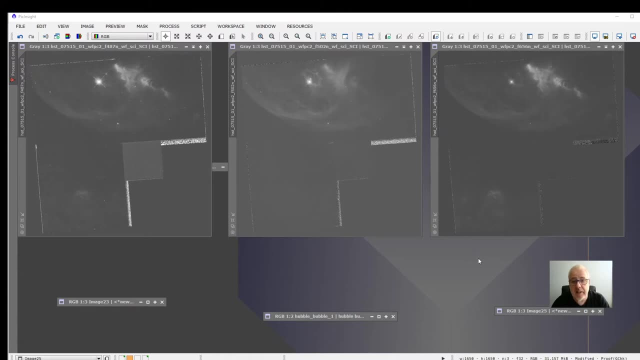 and then you simply press fetch hla data and you'll find that the the files are downloaded to the, the folder that you you've selected on your machine. as i said, these files are in fits formats, so if you've got pix, insight or any other processing software that deals with the fits, 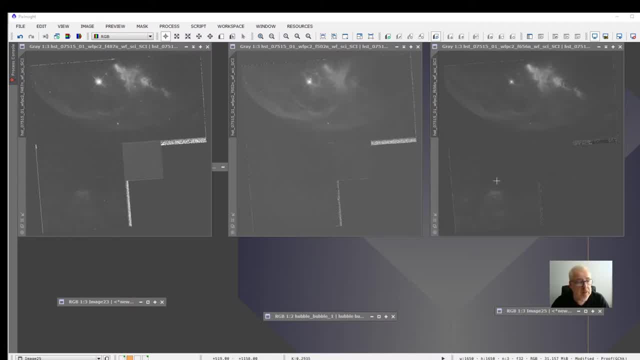 format, download them or download them straight away into the program and perform um a stretch on them, um so that they're they're non-linear and uh, as you can see here, that's exactly what i've done with each file. now the files are integrated files, they're, they're basically all the files have been calibrated, they've been. 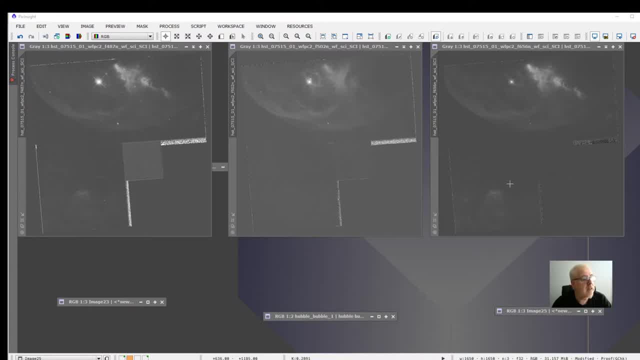 calibrated for bias, darks and flats. so what you've got is an integrated uh image from the raw data for each filter, so there's no need to stack anything. that's been done for you and it's been calibrated, so you simply got the calibrated stacks for each filter here if you haven't got pix insight. 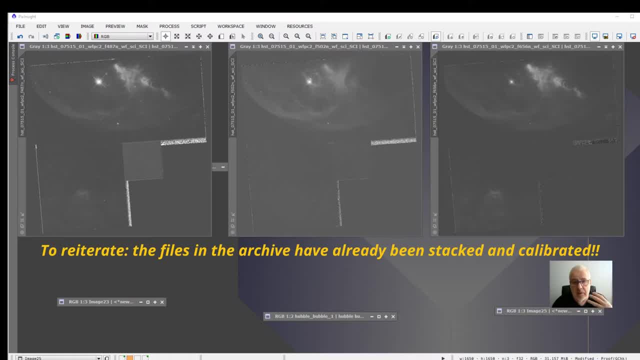 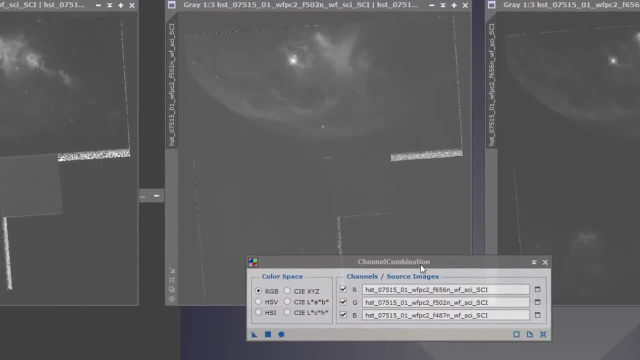 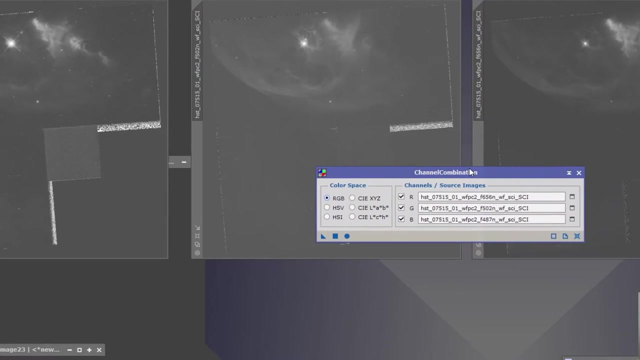 you can. you can use uh, photoshop or or something similar, but first you have to convert the fits fits files into tiff files, and i'll show you how to do that in a minute. but first let's just show you what happens in tiff files, pics in sight. so, just like you would normally do, to combine monochrome images into a color image, 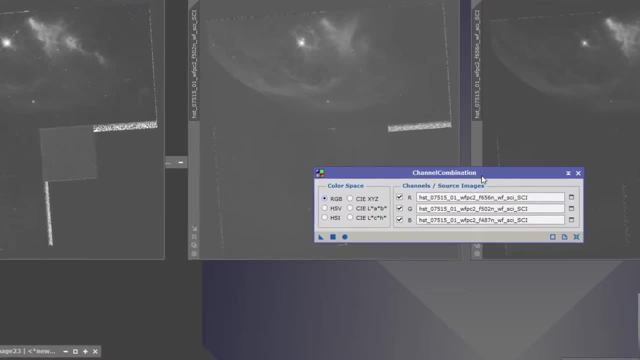 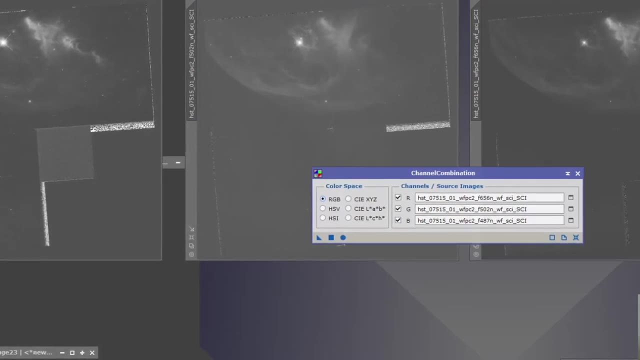 whether it's broadband or narrowband, you select the different files and allocate them to, or map them to, particular red, green or blue channel. now, in this case, it's the the filters are very different from the normal kind of filters that we're used to, so what? the way we do it is simply. 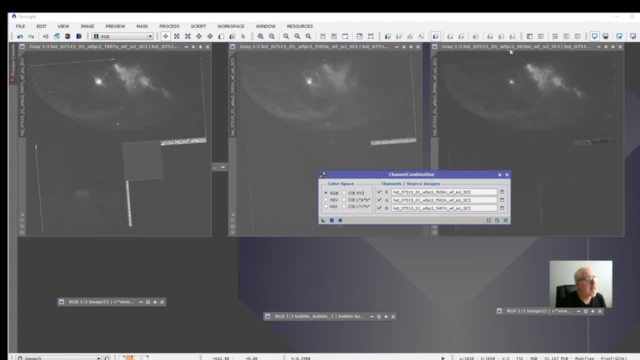 take the longest wavelength. so 656 nanometers is clearly a longer wavelength than 502, which is longer than 487. so take your longest wavelength, in this case 656, and allocate it to the red channel. okay, 502 is the next longest. allocate that to the green. 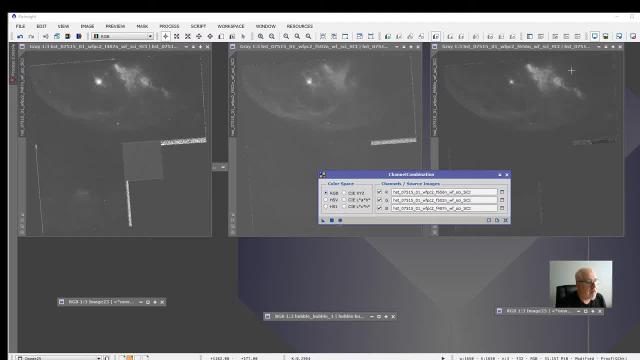 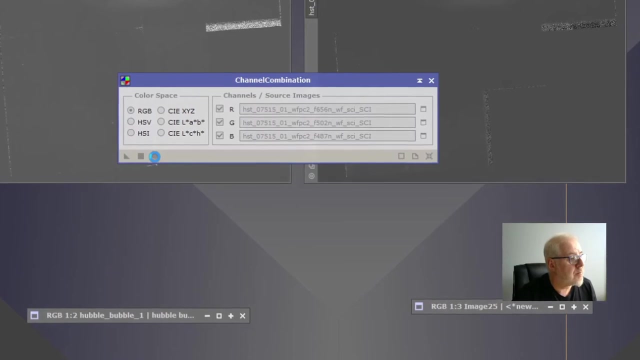 and four, seven to the blue. so, just to reiterate, the highest number of the filter goes to the red, the middle one goes to the green and the smallest number goes to the blue. okay, and once you've done that, just as you would in any other processing and pics in sight, let the thing do its, its job. 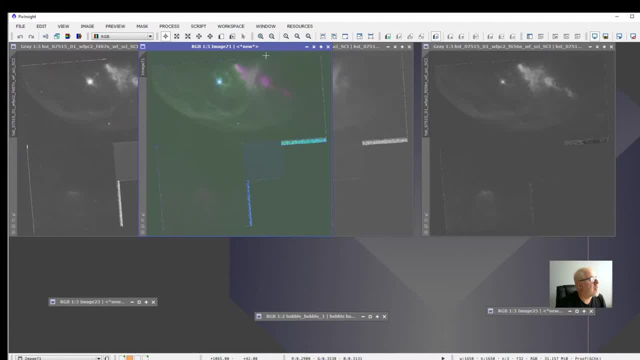 and here we've got a color image. now we can use dynamic crop. obviously, this is which is what i've done, and you can do the usual type of processing that you're used to doing in your narrowband or broadband image processing. so what i've done here, as i say i've, i've performed a dynamic crop and 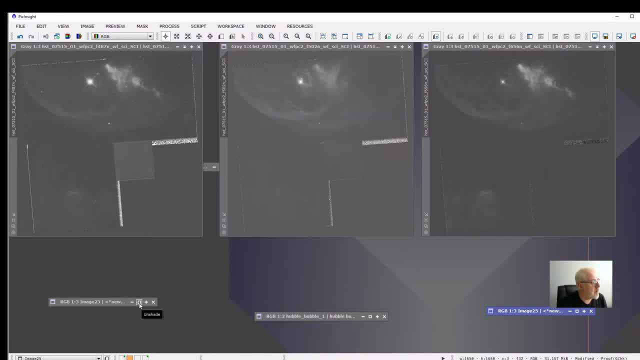 i've done various things and you can see that in here it's the same process, but you can also use it on the other side as well. I've ended up with, dare I say it, two different sort of colour palettes, and I eventually decided. 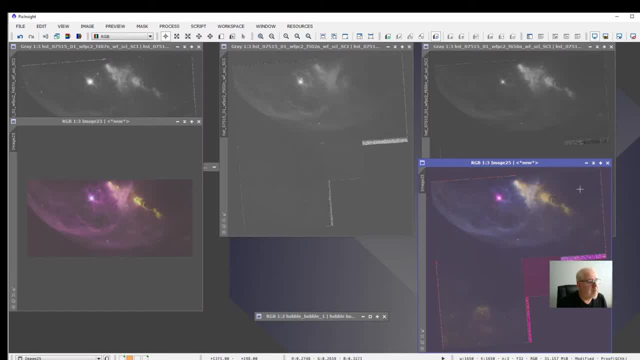 on this one here, just simply because I thought it looked better than that. I don't know what you think. Maybe I got it wrong, I don't know. Anyway, I decided to go for this image here, obviously with a dynamic crop, etc. And this is pretty much what it looked like once I'd 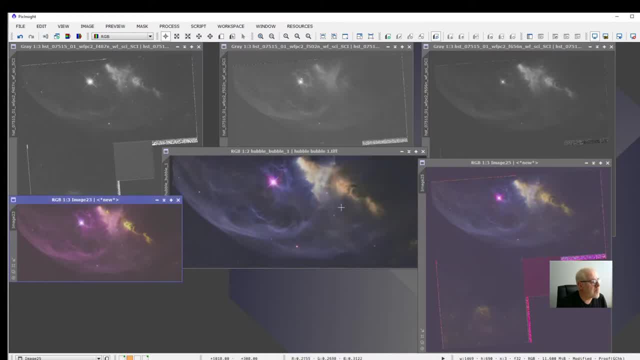 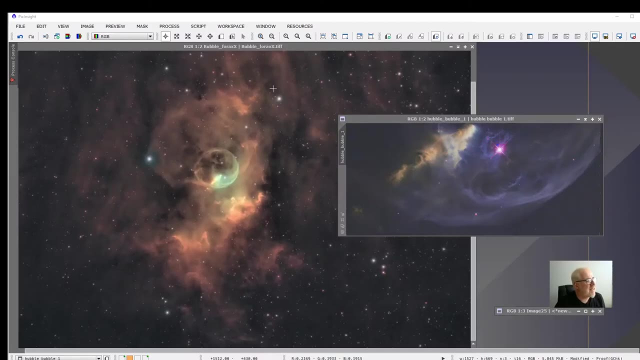 finished toying about with it. So, yeah, we have a not bad image at the end of the day. Again, we'll come back to that in a second. Here's the image of the bubble nebula I took about a year ago. It's a narrow band image. I used the 460mm. 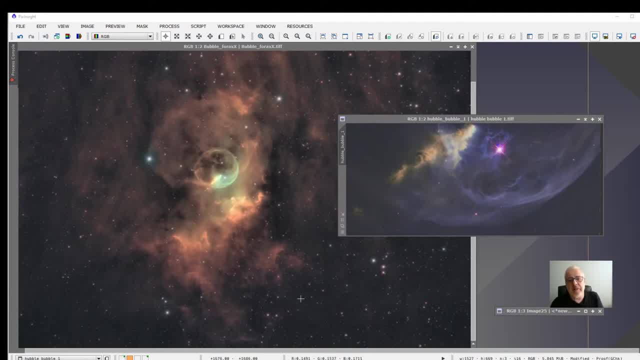 It's a 460EX with Sulfur II, Oxygen III and Hydrogen Alpha filters. The 460EX is a monochrome camera And I processed it using dynamic blending, using the 4AX method that I've talked about in a previous video, when I was looking at the Optolong filter. There's no contest really. 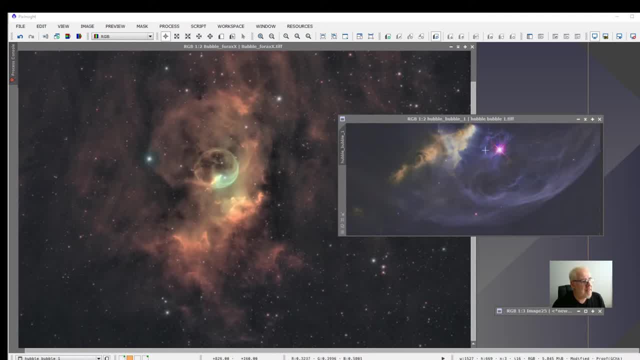 is there, I mean. so what I've done is I've re-orientated the Hubble image that I've processed, and so it sort of corresponds to the orientation in my effort. There's no contest, like I say, but what we've got here is this image, here is in this region, here You can see that stars, here. 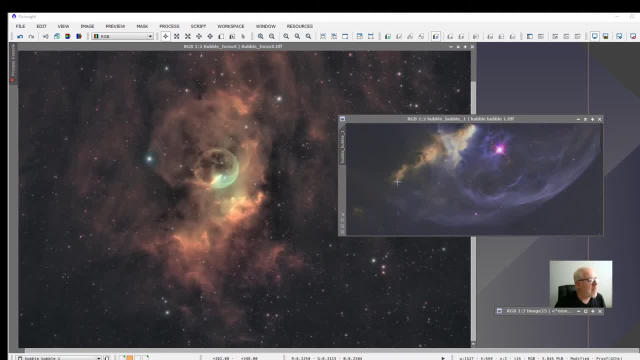 And we've got this little cloud, or nebula, complex, gaseous, complex, here, obviously in much more detail, Interesting, Interesting, Interesting, Interesting. nonetheless, isn't it A different kind of colour palette, but you get the idea. 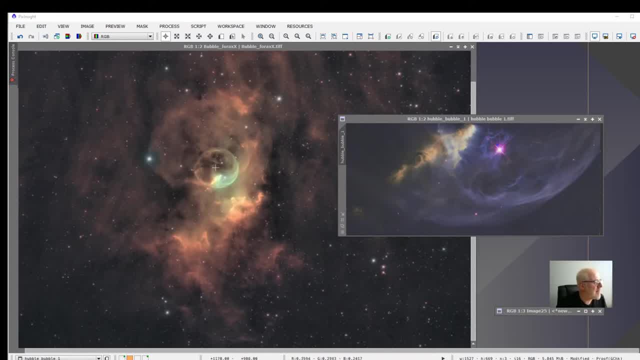 It's incredible to actually look at this in more detail And, as I say, some of the- well a lot of the images in this archive have never actually been published before. I don't recall seeing this one here being published, So it's very interesting just to see the difference. 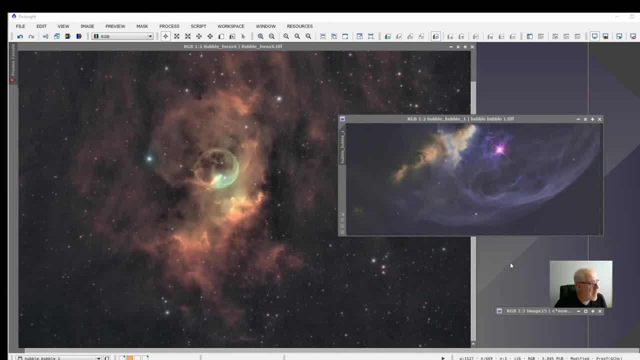 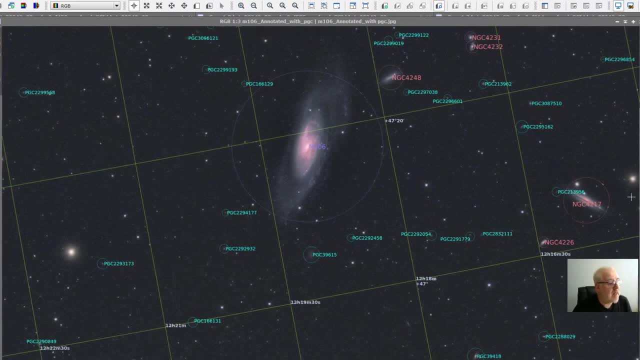 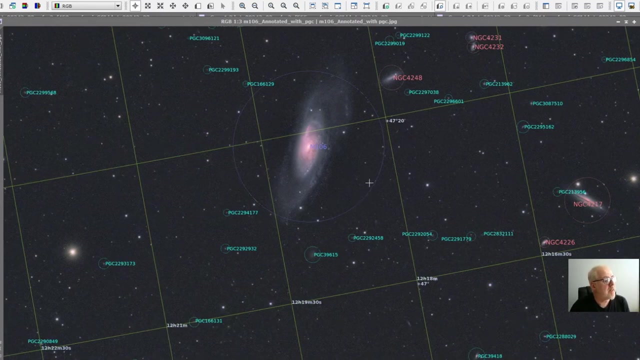 A bit of interest, a bit of fun, really. The next object or Hubble image I thought I'd download relates back to, again, a video I did recently regarding annotating deep space objects in your images, And this was the one regarding Messier 106 that I showed you recently. But what I thought might be a bit of fun is: 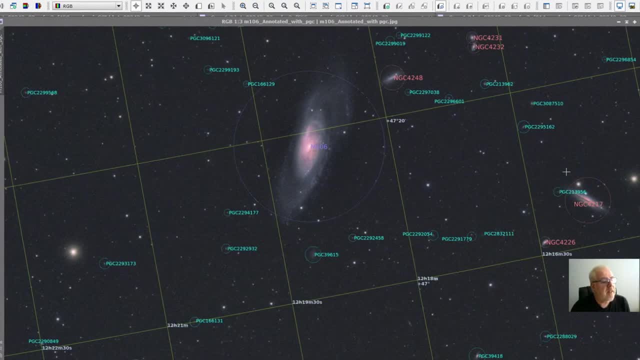 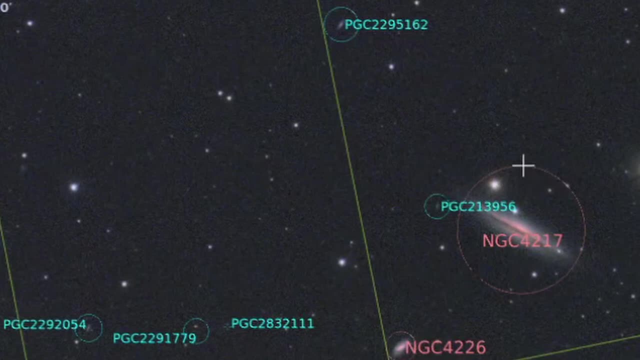 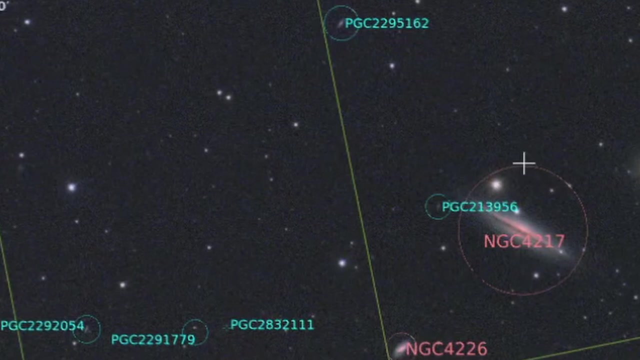 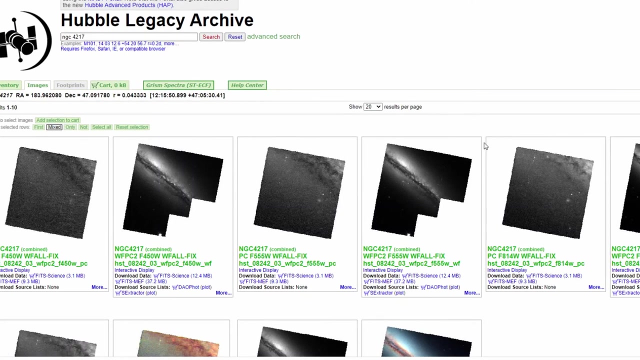 this galaxy, Galaxy here, NGC 4217.. Just to see what the Hubble telescope makes of this image. So I went ahead and downloaded the files relating to this particular object, Just as before. again, you put the object in, you search for it and it will come up with a number of. 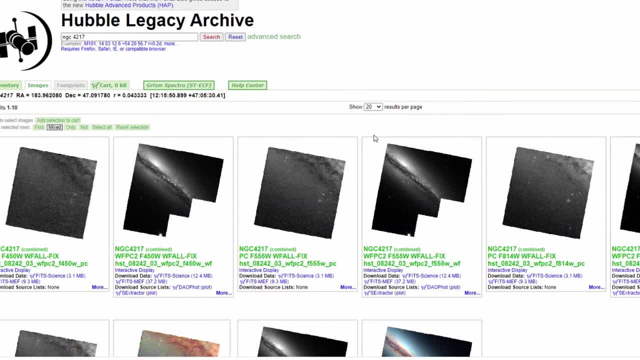 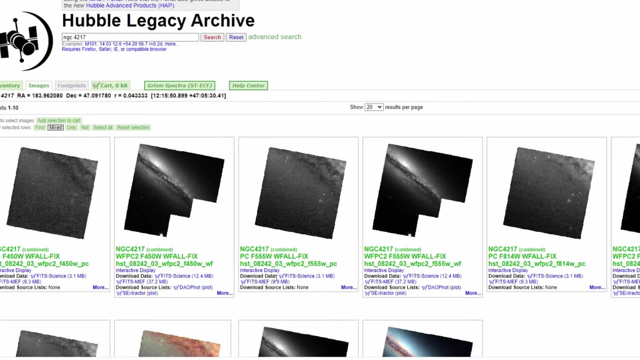 thumbnails relating to the image session Relating to this object. So again we can see here there's the proposition number, there's the visit number. It's taken with the Wide Field Planetary Camera 2.. This one was taken with the Wide Field Planetary Camera 2 as well. 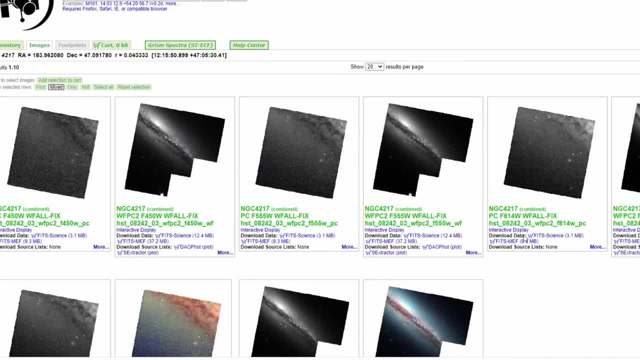 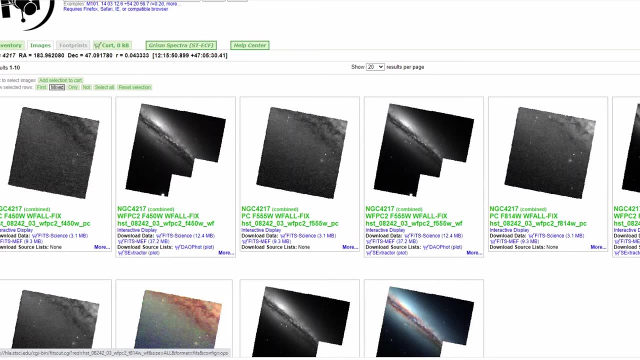 And on it goes. So again, what I've done here is I've downloaded one, One that corresponds roughly to the blue region of the spectrum, One that roughly corresponds to the green And one that roughly corresponds to the red. Okay, 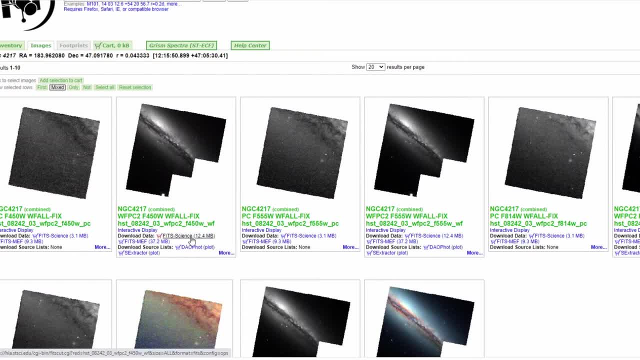 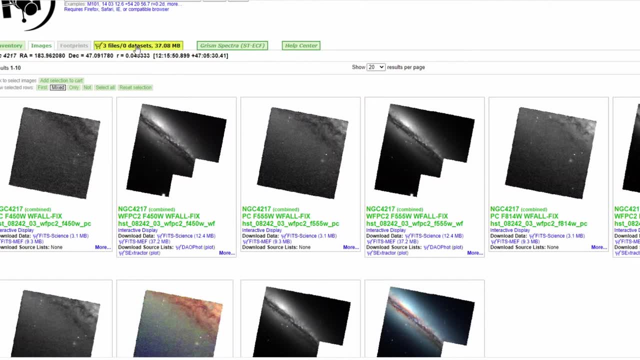 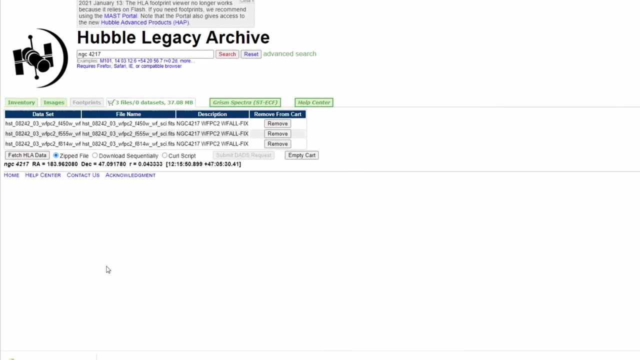 So again, just gone through the usual Click on the Science tab And they're all added to the cart, Ready for download. And again, all you have to do is click on the Fetch, The Fetch HLA data, And everything's downloaded. 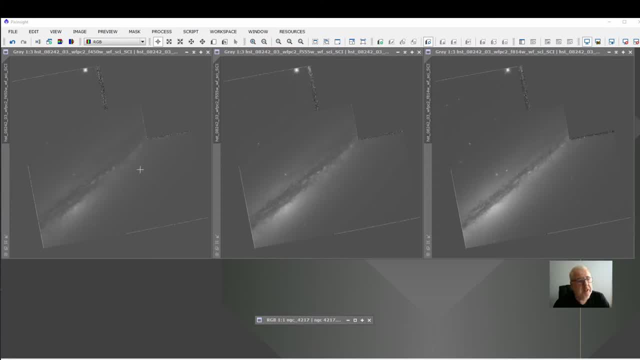 So again, you can see the stealth bombers' shapes in the different windows relating to each different filter. So here's what's going to be in our red channel, Here's what's going to be in our green channel And here's what's going to be in our blue channel. 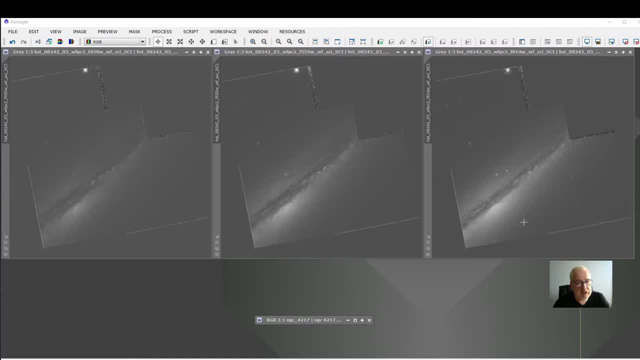 And again, I've stretched them using histogram transformation And applied some curves transformation to them as well. And just like the last time, the last image, I've also applied a dynamic crop to each And mapped them to the relevant color channels. 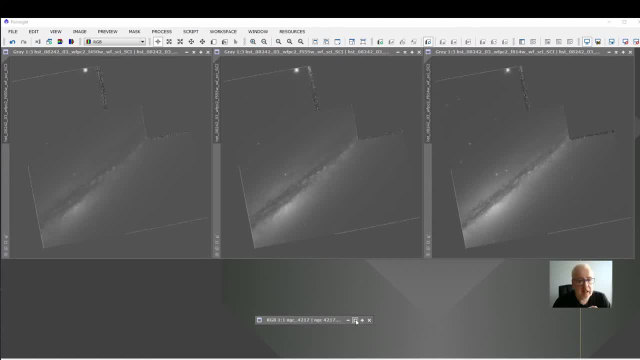 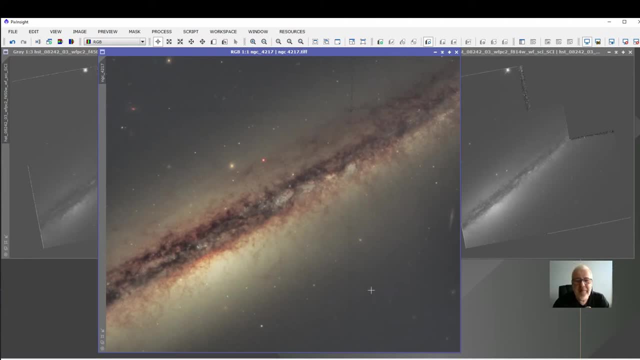 And had a bit of a play, And this is what I came up with. It's really nice, isn't it? I love to save. I love to save. This is an image I've taken, But that would clearly be lying. 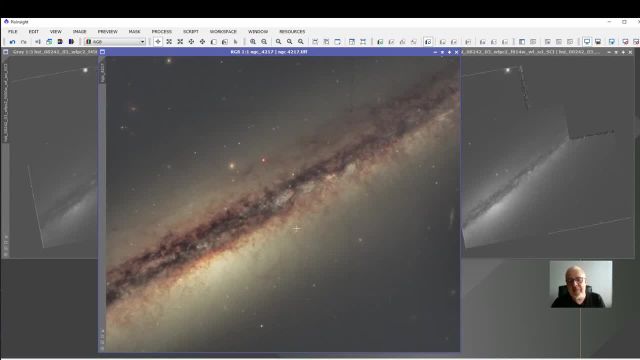 Yeah, So it's. obviously they've not imaged the whole galaxy, But what they've done is taken on the dust, the dust lane. Now you can see there's a few artifacts in this image, And that's to do with the camera itself. 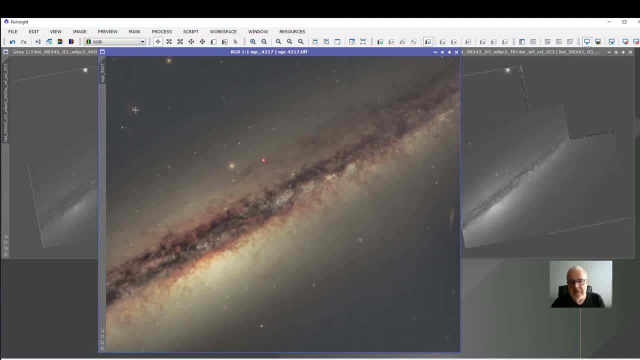 That's to do with how the chips laid out, Or the different chips in the camera laid out, And I'm going to show you a quick fix how you can get rid of these quite easily. But first let's see how that compares to the image of this galaxy that was taken in the one that I imaged. 106 in. 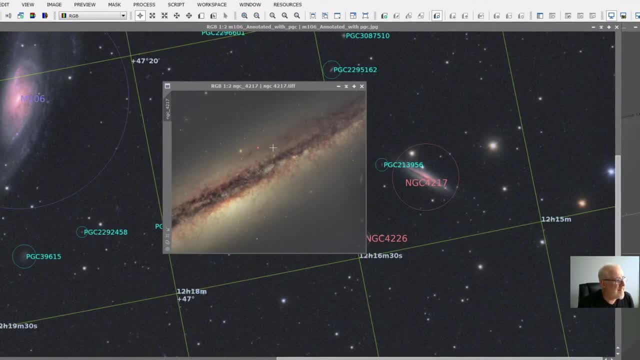 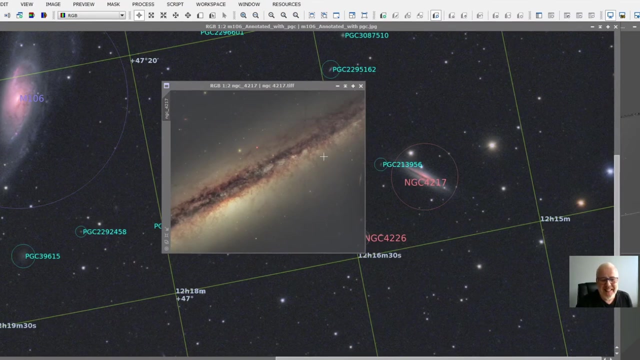 Well, here we are Again. look at the detail in it. It's absolutely incredible. Having said that, you know my image isn't that shabby, I don't think, But obviously nowhere near the detail that this gets. 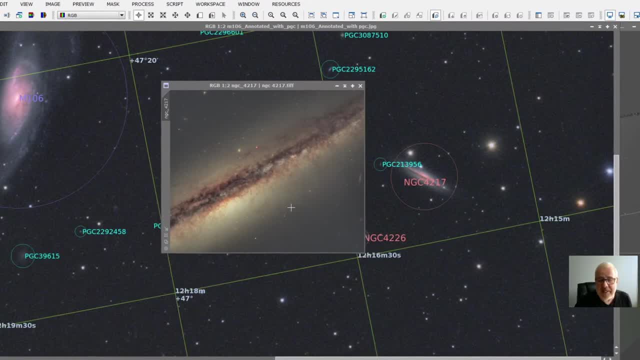 So, again, it's just an interesting exercise, I think, particularly if it's an object that you're not too sure of Or you know, in this case NGC 4G, NGC 4217.. It's not the most well-known galaxy as well, to me anyway, 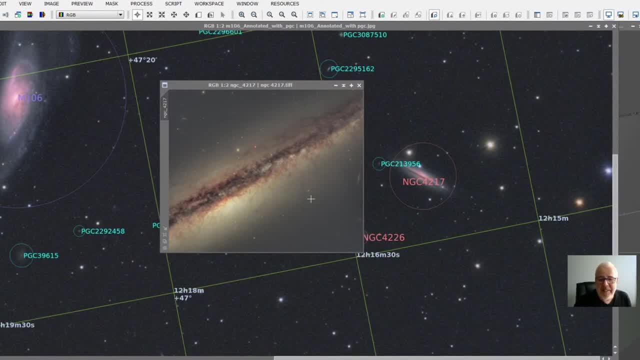 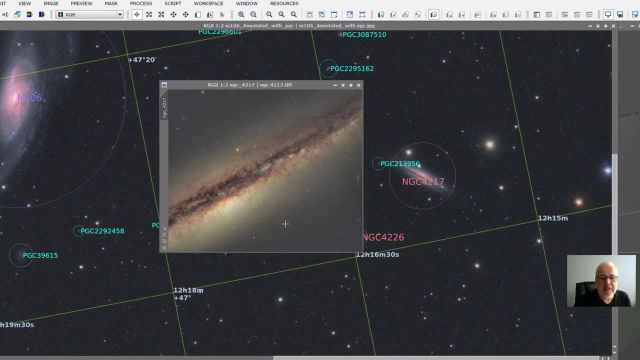 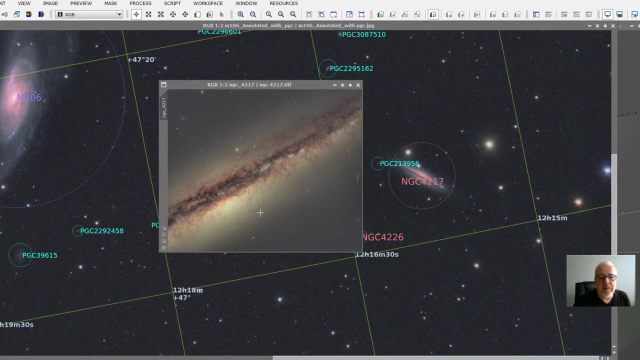 But it's just nice to see an image of it that Hubble's taken Again. I'll show you how to get rid of these artifacts that do occur, Particularly in the Wide Field Planetary Camera. 2. The old camera that was replaced in 19..2009, sorry. 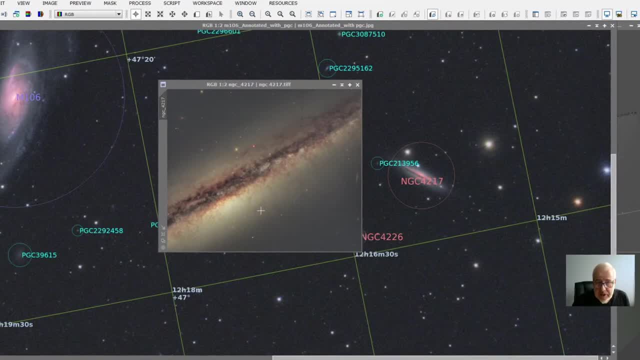 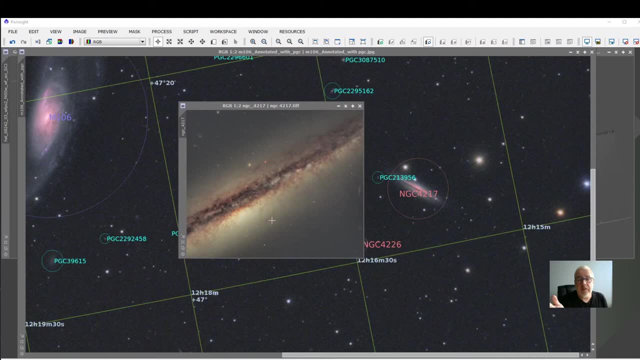 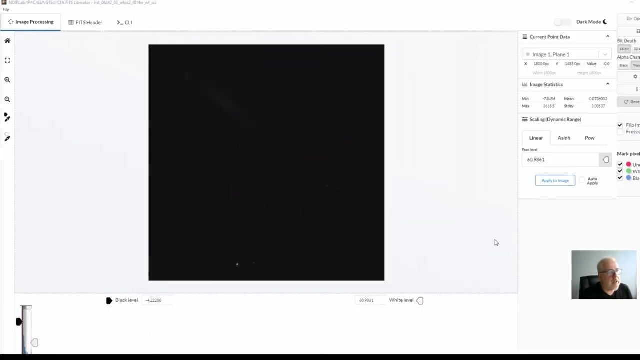 I'll show you that in a minute, But first, as I said, I've been using PixInsight here. I'll show you how to convert the files into TIFF files so that you can use them with Photoshop. To do the conversion, so that you can use your files in Photoshop, you have to download a particular piece of software called FitzLiberator. 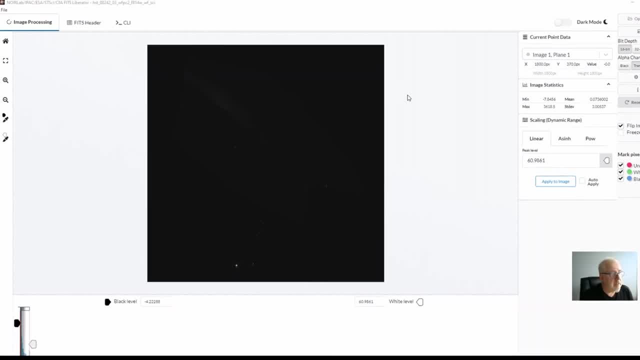 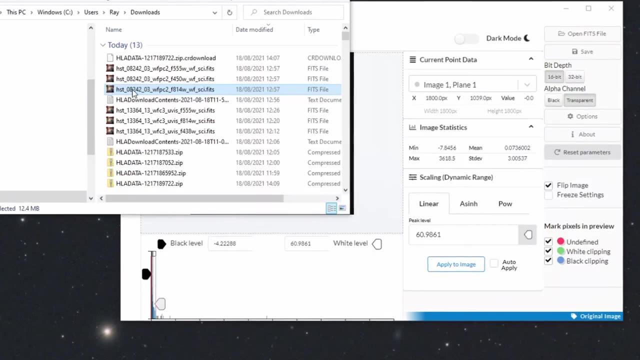 It's free and it does exactly what it says. It basically converts Fitz files into TIFF And it allows you to stretch them before obviously converting them, So you can use them in a non-linear form. I did this particular file, which is the 814 filter, into FitzLiberator. 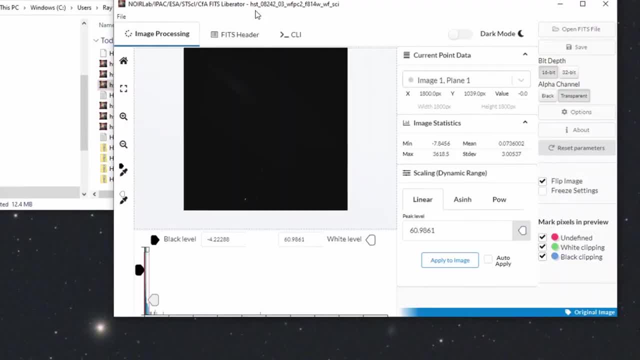 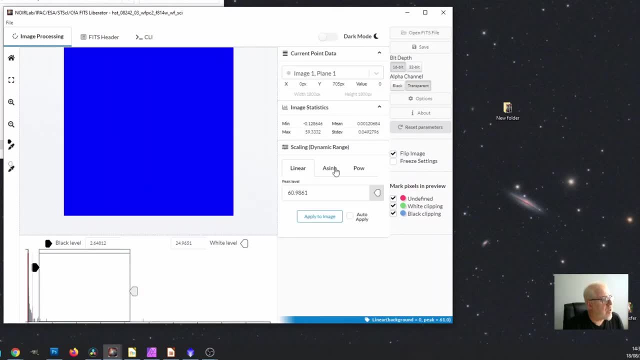 You can see it's nicely loaded up here. Once your file's loaded, you need to change the dynamic range scaling to to this particular configuration here: Ace and H. Okay, And what you'll be presented with is this little Curves, the dark and white point box. 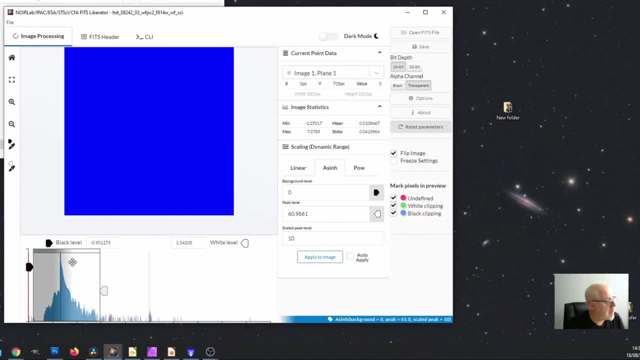 And what to do is simply move it over to the peak of the image like so, And you'll start to see your image getting stretched, And It's really just a question of playing with the dark and white points to get the best. 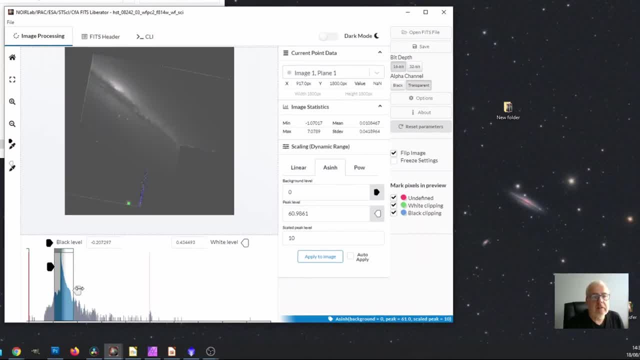 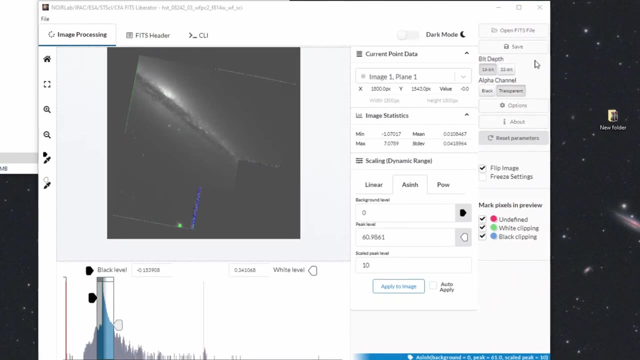 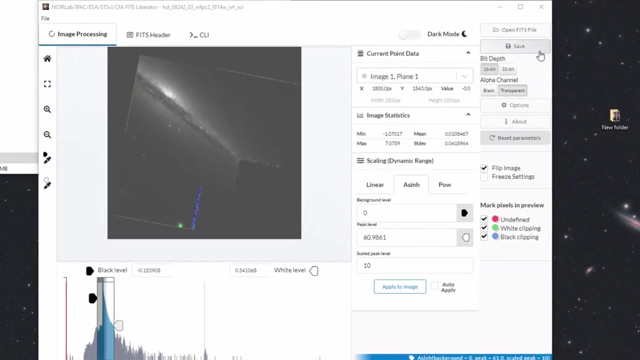 To get the best picture you can, or image you can For later manipulation, So that looks reasonable. And again, once you're happy with that, simply press save into a particular directory that you want to save these files to for use in Photoshop later. 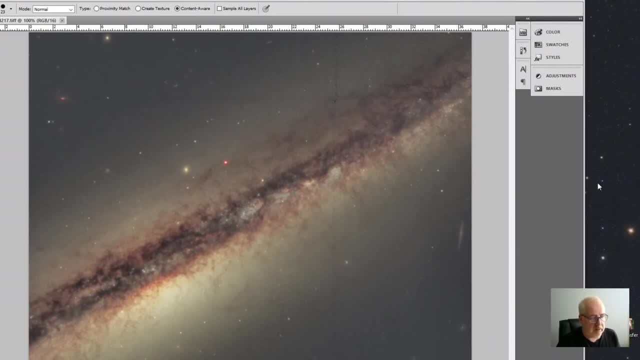 Here I've loaded up the image of NGC 4217.. And, as you can see, it's got these kind of nasty little artifacts, Again due to the camera construction And you probably, If you use Photoshop for your Processing. 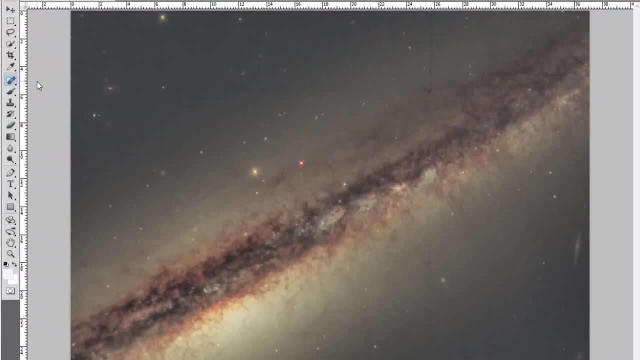 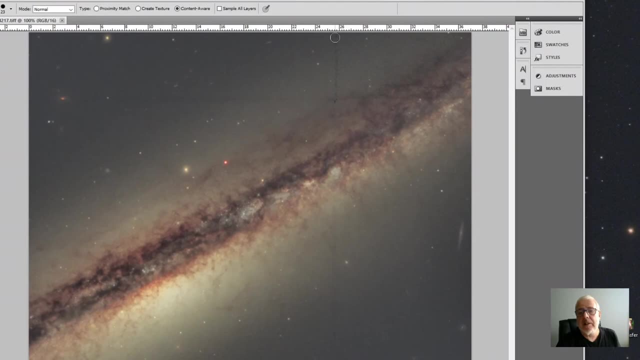 I'm more aware of this feature than I am, But essentially it's called the healing tool, if you're not, And basically it samples the background and replaces the artifacts simultaneously. It's great. So here you can see, Obviously, a join and a mosaic of some sort. 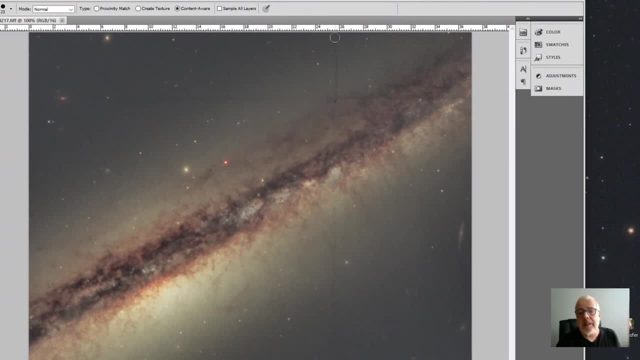 It's where the different chips, as I understand it, are physically linked. But simply drag it down And it's magically gone. And again, if we simply move it across here, Gone And great, Gone, Wonderful. Obviously, it should take a bit more care of it than I've just done. 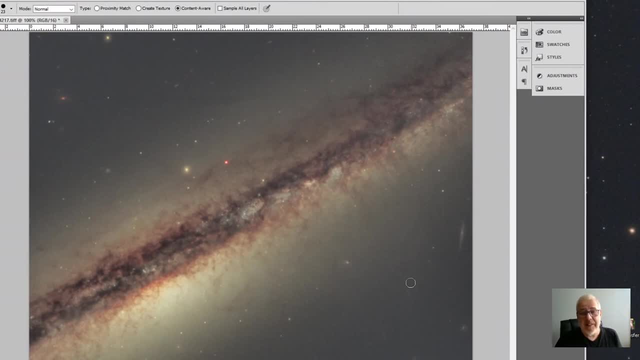 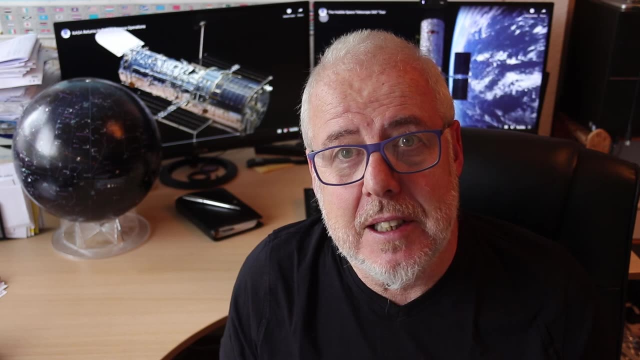 But it cleans the image up nicely. Well, folks, That's the end of that video. I hope you found it interesting And, as I say, it's all free to use and download. You can access a lot of material that's never been published before.